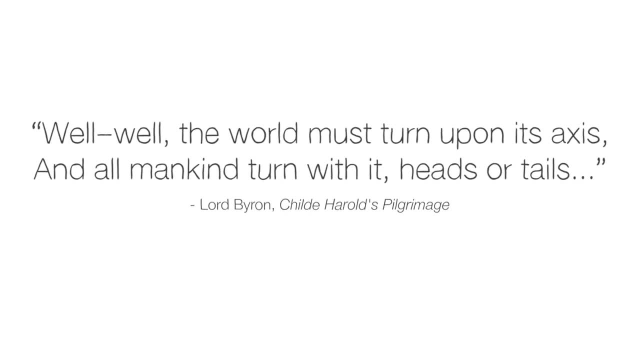 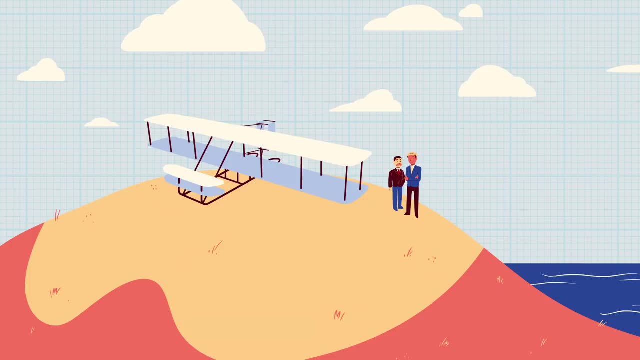 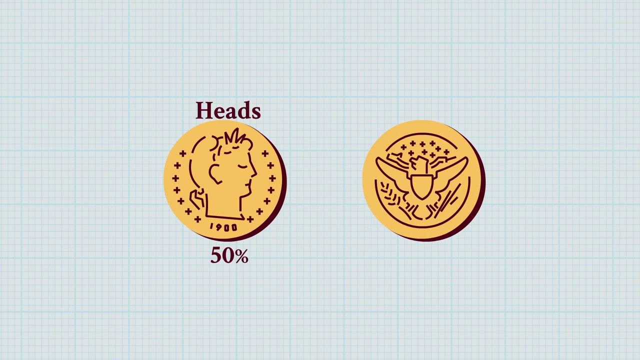 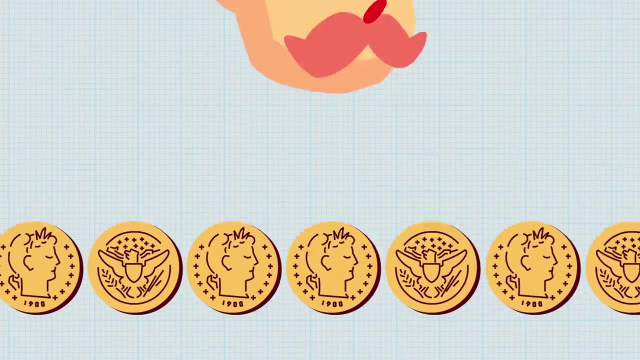 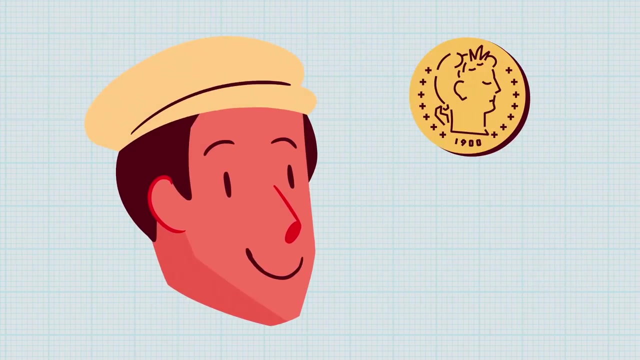 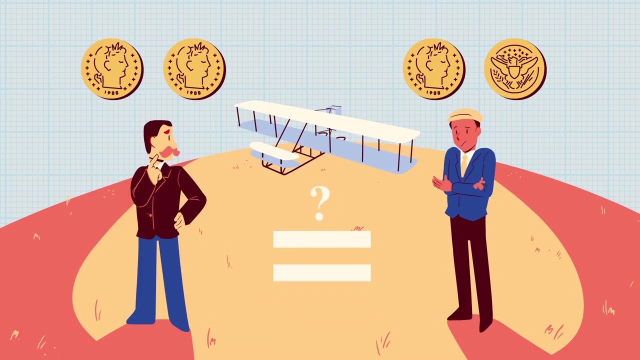 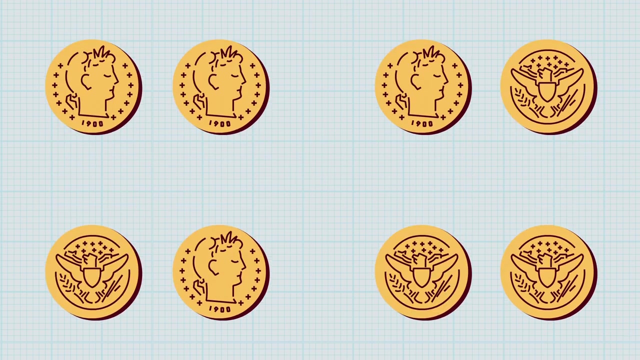 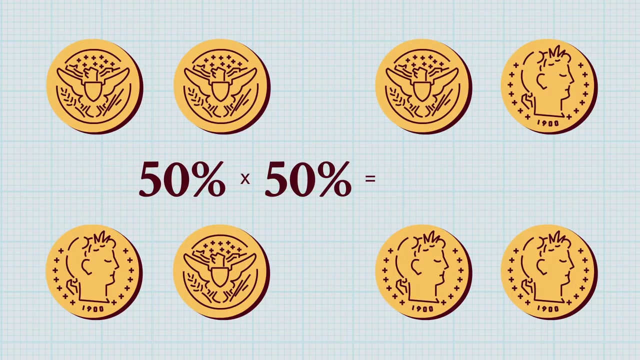 Thank you for watching. Would each brother still have had an equal chance to be the first in flight? At first, it may seem they'd still have the same chance of winning. There are four combinations for two consecutive flips, and if you do flip a coin just twice, there's an equal chance of each one—25%. 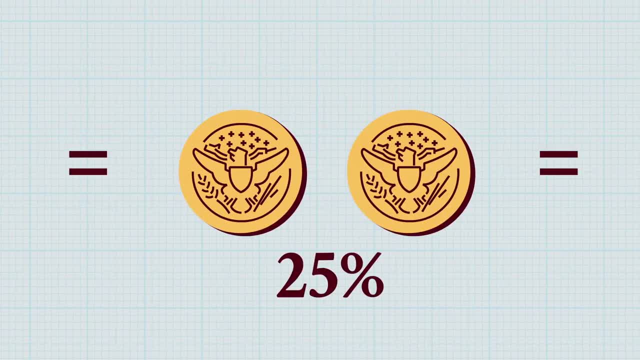 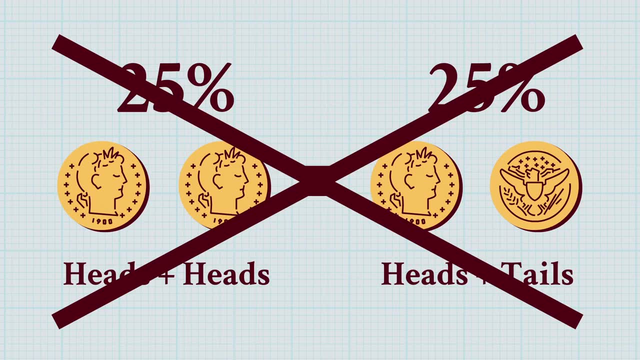 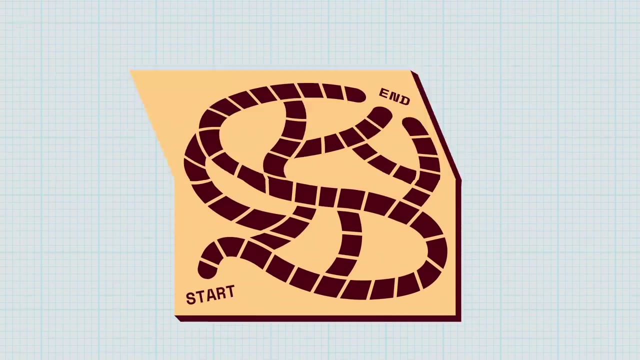 So your intuition might tell you that in any string of coin flips, each combination would have the same shot at appearing first. Unfortunately, you'd be wrong. Wilbur actually has a big advantage in this contest. Imagine our sequence of coin flips as a sort of board game. 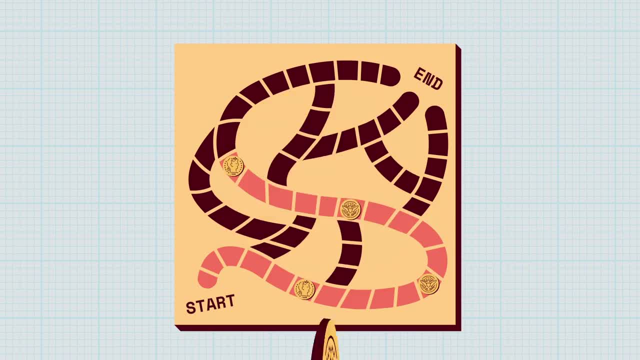 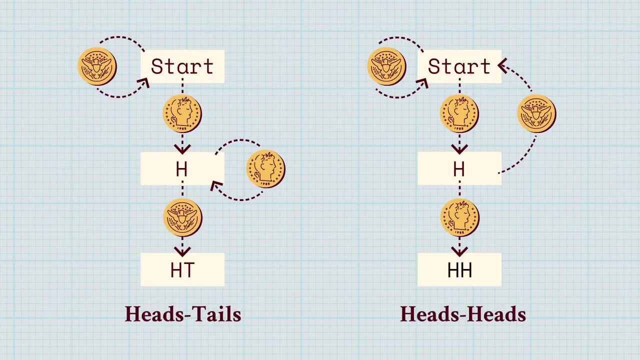 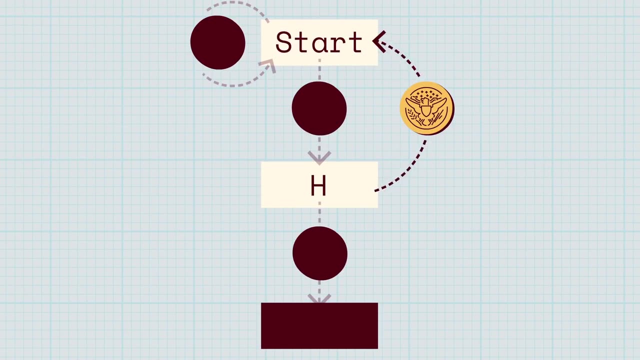 where every flip determines which path we take. The goal is to get from start to finish. The heads-tails board looks like this and this is the head-head board. There's one critical difference: Heads-heads has a move that sends you all the way back to the start. 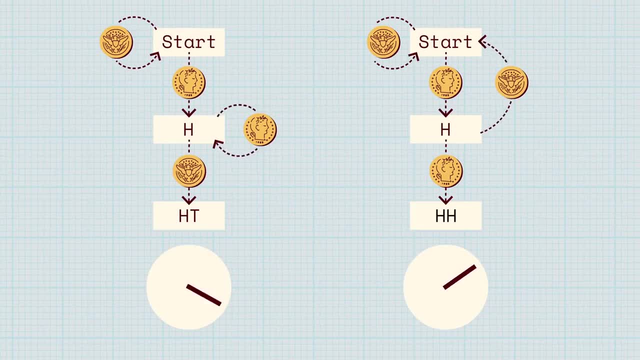 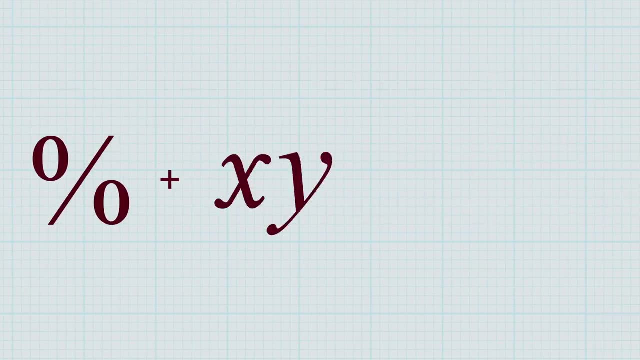 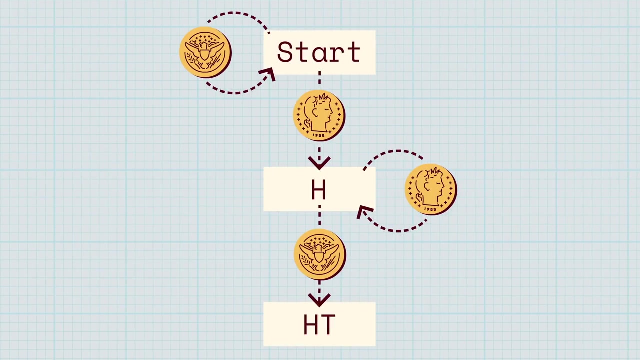 that heads-tails doesn't have. That's why heads-heads takes longer on average. So we can demonstrate that this is true using probability and algebra to calculate the average number of flips it would take to get each combination. Let's start with the heads-tails board. 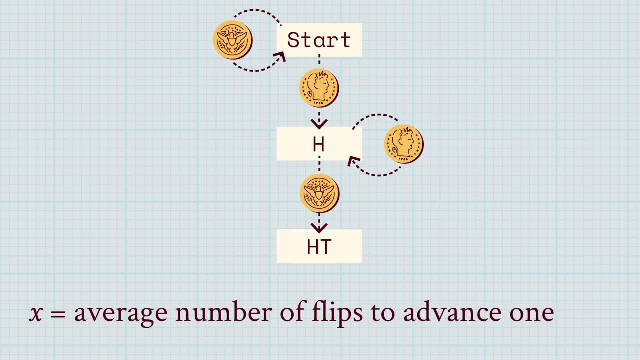 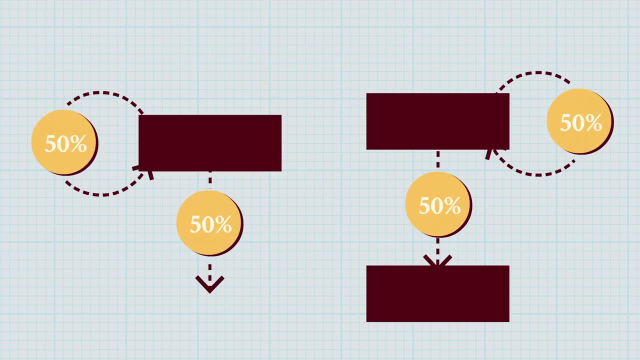 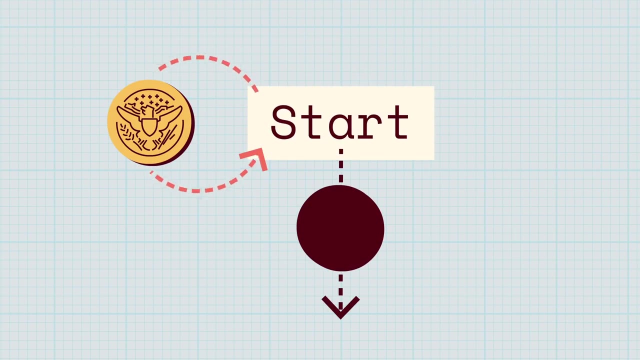 and define x to be the average number of flips to advance one step. Focus only on the arrows. It has two identical steps, each with a 50-50 chance of staying in place or moving forward. Option 1. If we stay in place by getting tails. 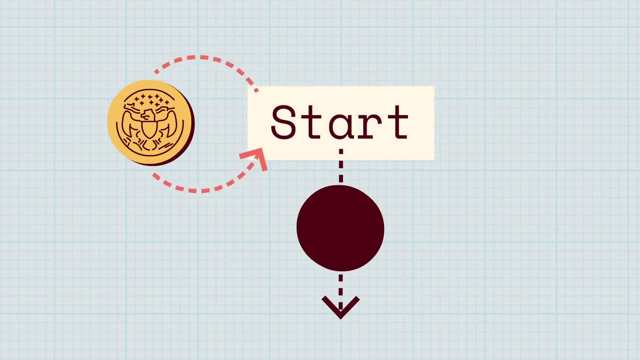 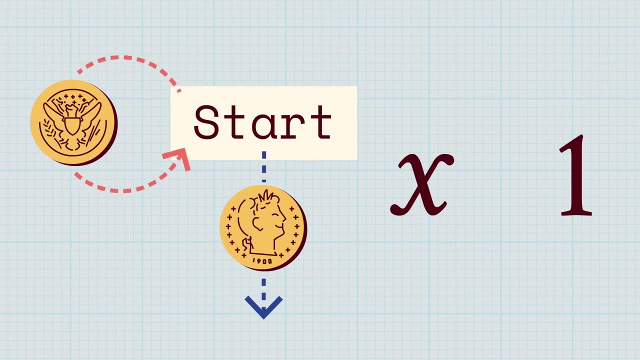 we waste one flip. Since we're back in the same place, on average we must flip x more times to advance one step Together with that first flip. this gives an average of x plus 1 total flips to advance Option 2.. 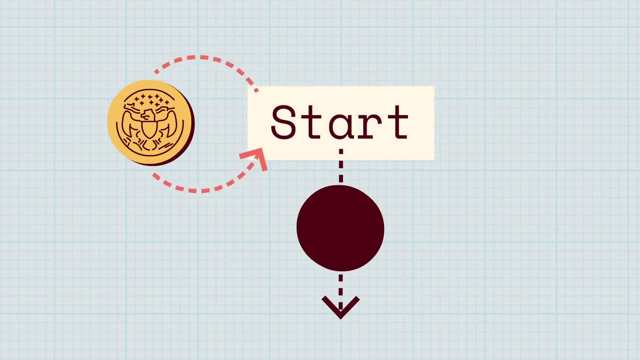 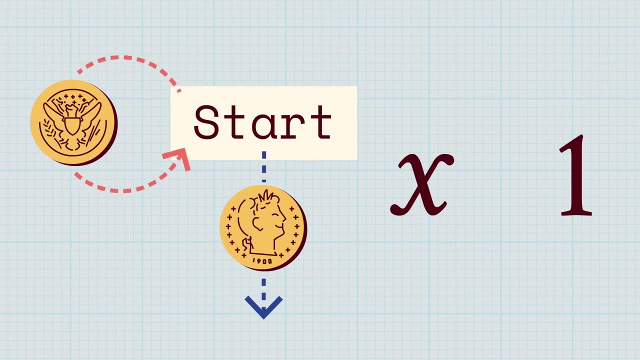 we waste one flip. Since we're back in the same place, on average we must flip x more times to advance one step Together with that first flip. this gives an average of x plus 1 total flips to advance Option 2.. 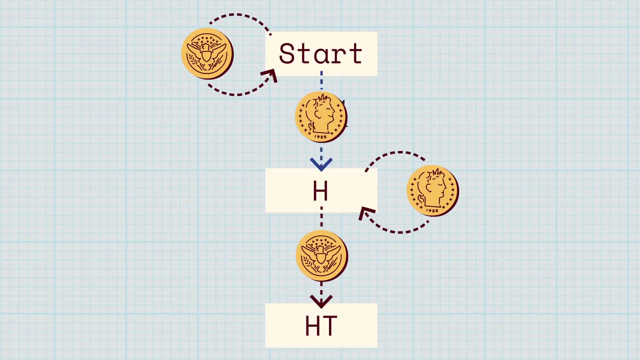 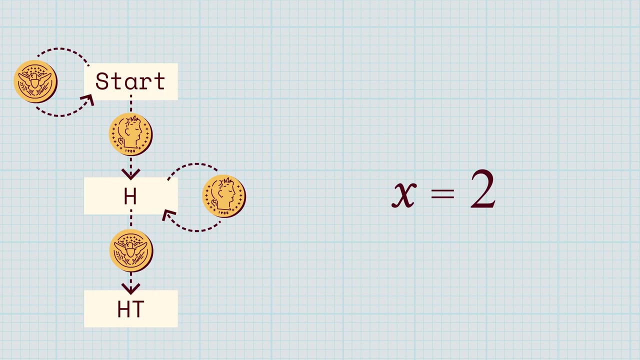 If we get heads and move forward, then we have taken exactly one flip, one total flip to advance one step. We can now combine option 1 and option 2 with their probabilities to get this expression Solving. that for x gives us an average of two moves to advance one step. 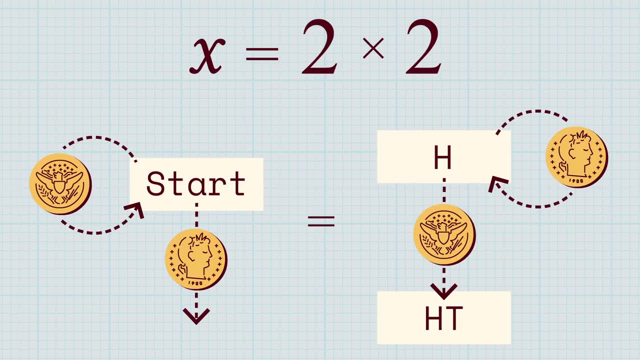 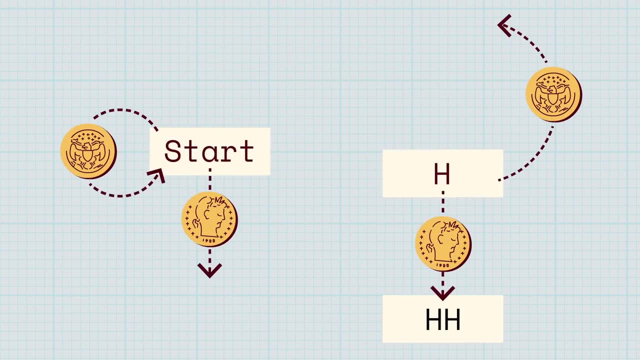 Since each step is identical, we can multiply by 2 and arrive at four flips to advance two steps. For heads-heads, the picture isn't as simple This time. let y be the average number of flips to move from start to finish. 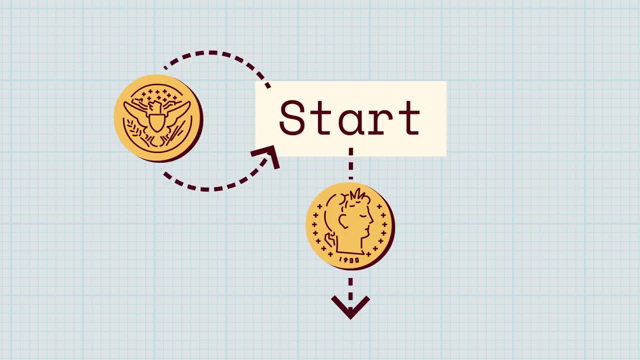 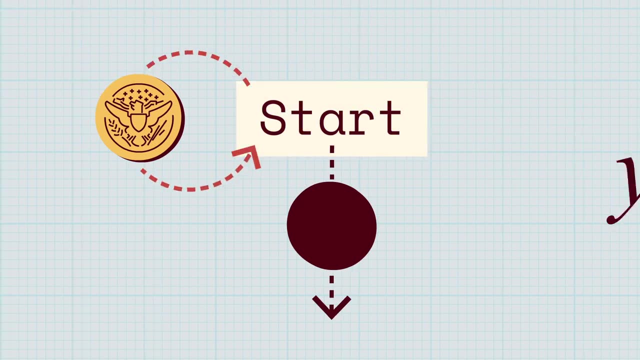 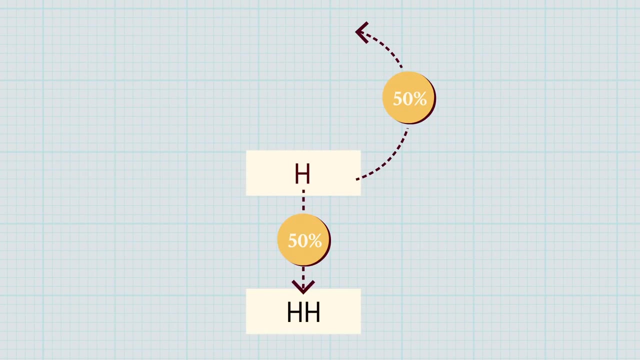 There are two options for the first move, each with 50-50 odds. Option 1 is the same as before: Getting tails sends us back to the start, giving an average of y plus 1 total flips. to finish In option 2, there are two equally likely cases for the next flip. 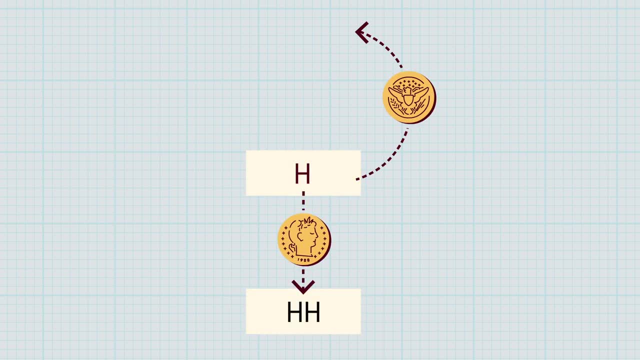 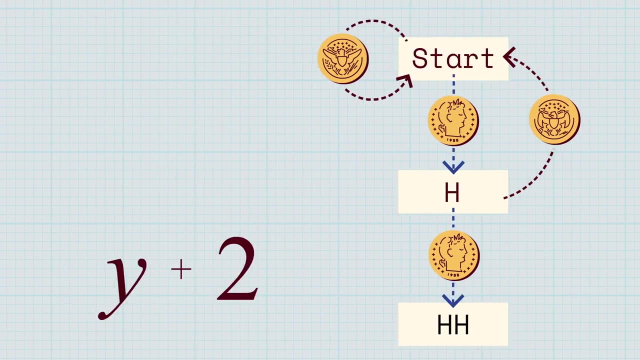 With heads we'd be done after two flips, but tails would return us to the start. Since we'd return after two flips, we'd then need an average of y plus 1 total flips to finish. y plus 2 flips in total to finish. 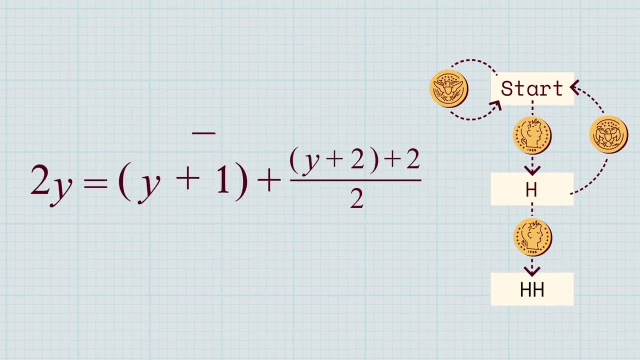 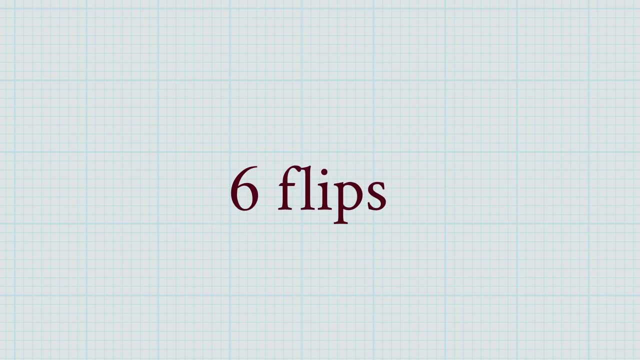 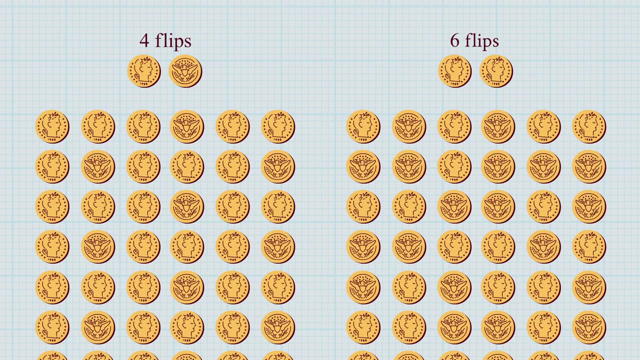 So our full expression will be this: And solving this equation gives us six flips. So the math calculates that it takes an average of six flips to get heads-heads and an average of four to get heads-tails. And in fact that's what you'd see if you tested it for yourself enough times. 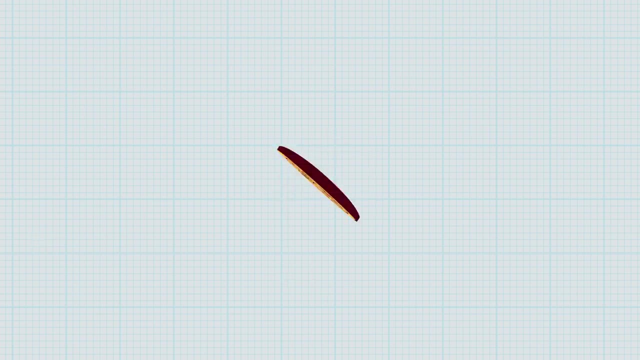 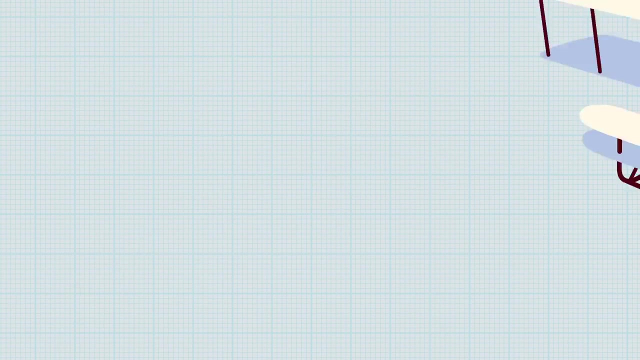 Of course, the Wright brothers didn't need to work all this out. They only flipped the coin once And Wilbur won. But it didn't matter. Wilbur's flight failed and Orville made aviation history instead. Tough luck, Wilbur.